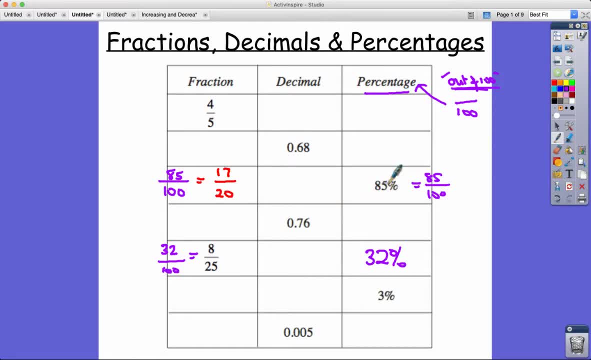 a random order, but I think you know we explain along the way. It's quite good. 85 over a hundred as a decimal is 0.85.. So, knowing that we can then start to use a bit of detective work and start to fill in a few more things, This is 0.85 and it's 85%. 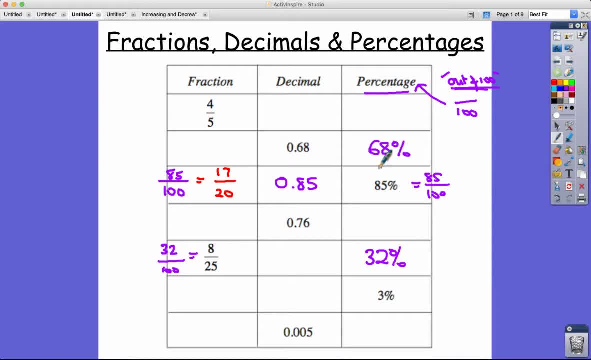 This is 0.68.. This would be 68%, wouldn't it? And this would be 76%, And this one here would have to be therefore 0.32.. Okay, Over here I can start to put in some fractions. 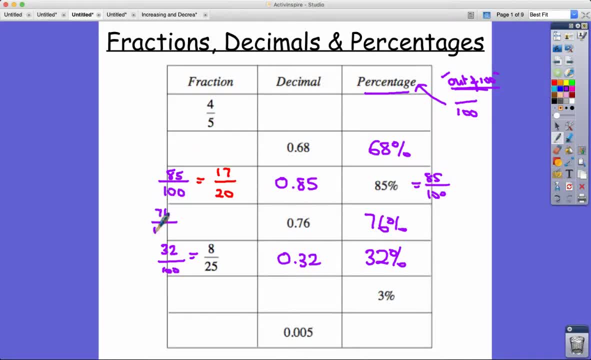 now as well. So 76%. well, that's 76 over a hundred. I think I can simplify that down to. let's think I can divide by four. I think First of all divide by two and get 38.. 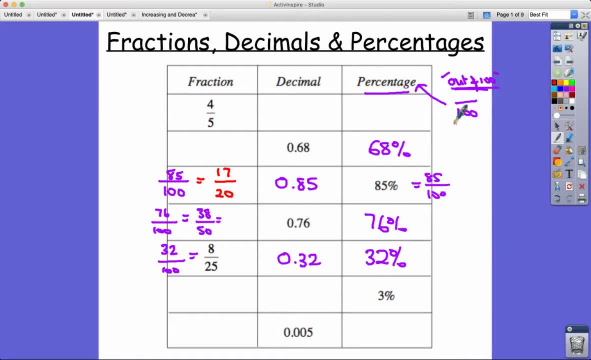 Over 50. And that can be simplified. again to my final answer of what? 19 over 25.. Let's do it for this one as well. We've got 68 over a hundred. That can certainly be simplified onto the simplest form, Again by doing a similar process: it's 34 over 50. Again, they're. 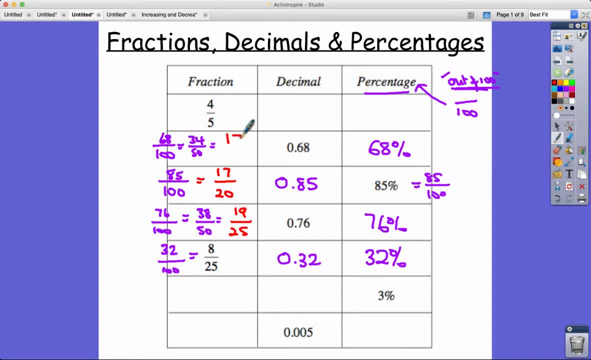 both even. So that would be what? 17 over 25.. Okay, So we're doing well This one on the top. let's do the top row now. Let's get this into hundredths. We'd have to times by 20. So this would be 80. And so it'd be 80%. And 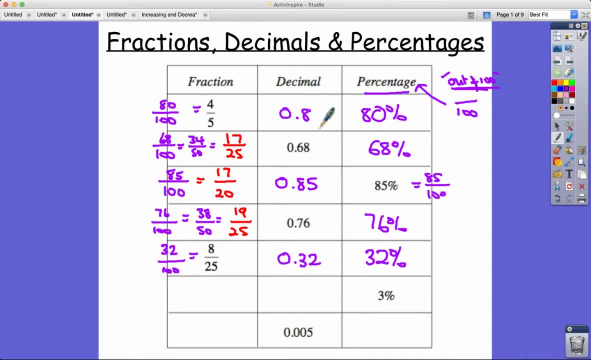 there's a decimal 0.8.. We could put zero on the end if we wanted to. It doesn't make any difference. 0.8 is fine though. Okay. So we've got those 3%. Now let's be really careful. 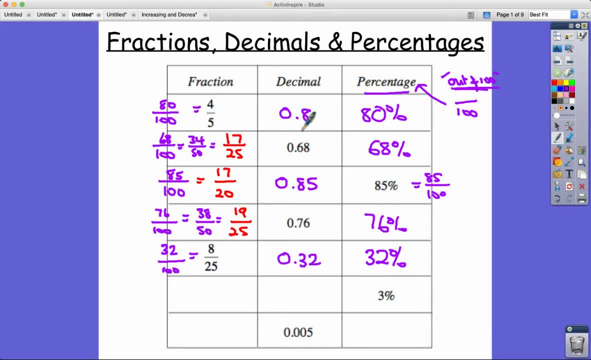 here It's not going to be. if we think about what 0.8 would be, it's going to be 0.8 over 80.. 0.8 is 80%. 0.3 would therefore be 30%. So it's not right. 3% is 3 over a hundred. 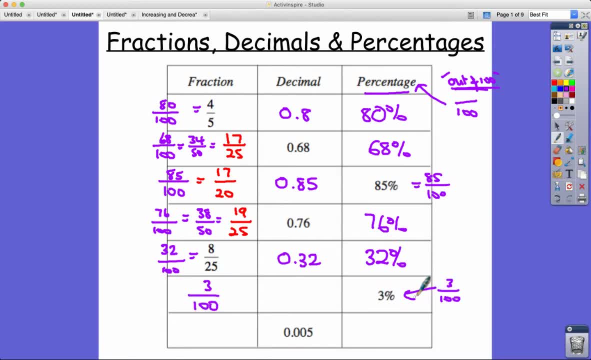 Well, actually, yeah, we can put that straight in, actually, because 3 is prime, We can't simplify it any further. So 3 over a hundred. And so you know- we talked about in a previous video on converting fractions to decimals that there's going to be two decimal places.